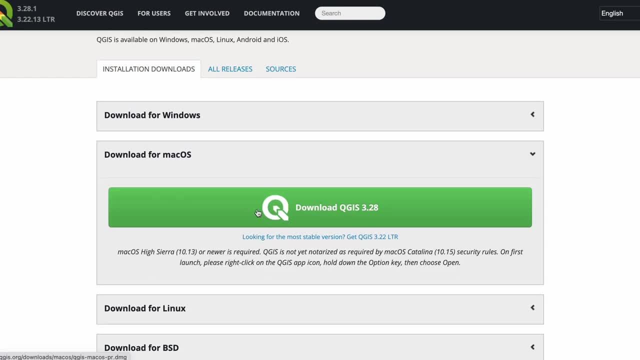 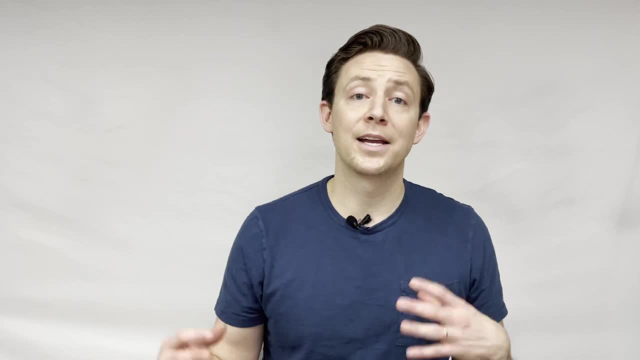 and anyone can use it. Plus, there's an amazing community of support around this tool. Is this still the tool that I use the most today? No, Would I change anything about the order? I learned this in No way. You can do everything from analyzing spatial relationships. reading. 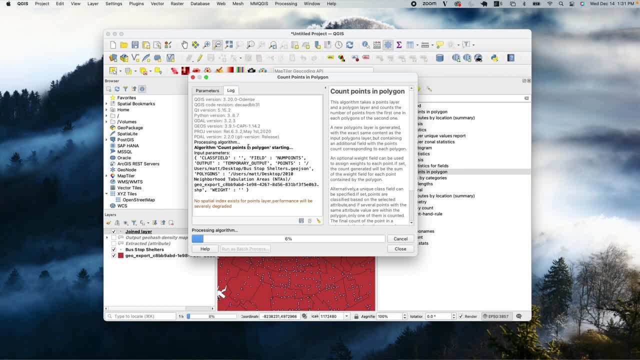 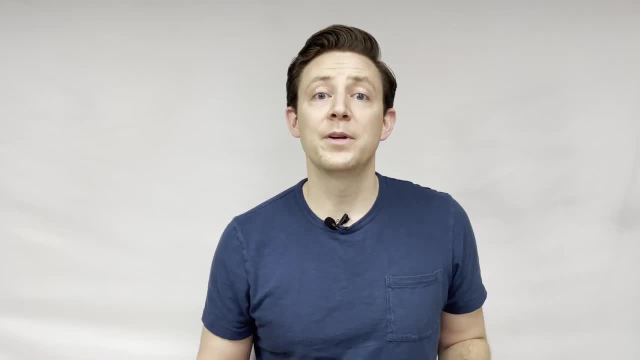 and analyzing raster files, even up to simple spatial statistical models, within QGIS, And if you can't find something that you need to do, I almost guarantee there's a plugin to do this. If you're coming from a more traditional GIS set of tools, this is a great place to start. 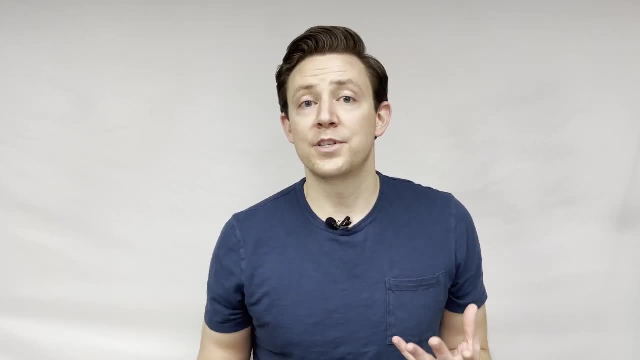 It'll feel super familiar and it's very easy to use. There are, of course, some limitations. with QGIS, You can't analyze super large data sets, Otherwise you might end up with a spinning wheel of death, like you see here. 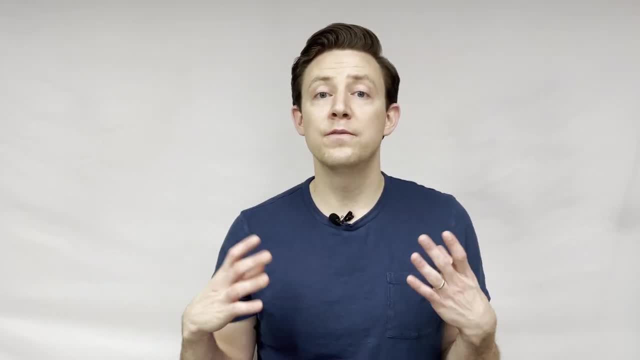 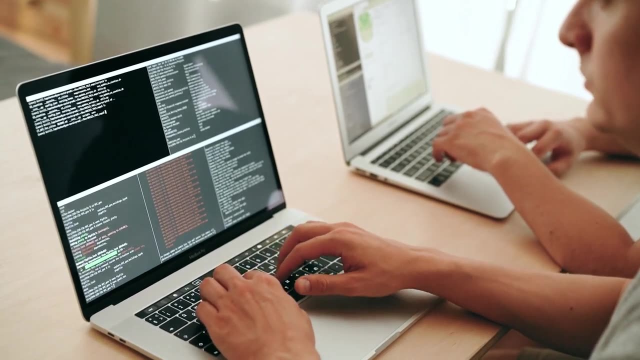 Once you've learned this, what's the next thing that you need to learn? So, once you've learned QGIS, it's time to move on to your next tool. Now you're going to need a programming language to do more spatial analytics and analyze larger data set. Previously, I said that Python was the best. 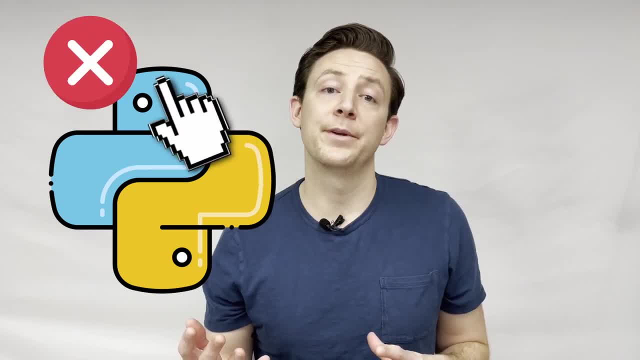 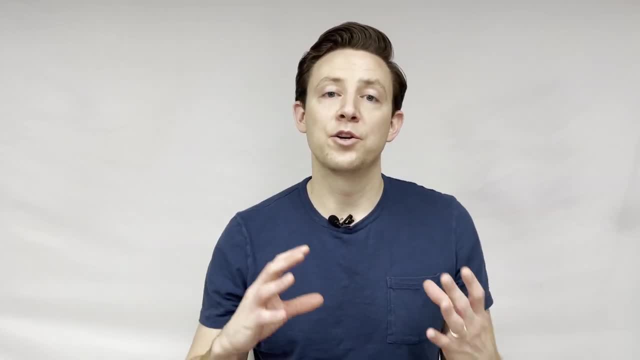 way to get started with this, and I'm actually going back and changing that recommendation a little bit. The next tool that I would learn is spatial SQL. So why SQL over Python? The answer is simple: The faster your ability to query, change and manipulate data, the faster your 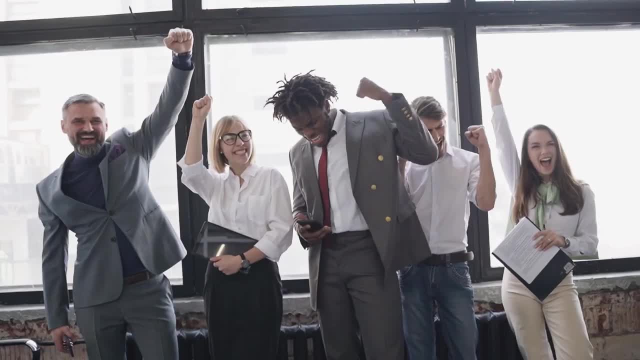 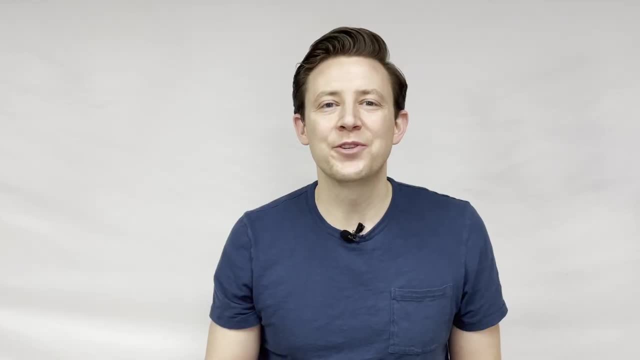 career will move as a spatial analyst. For me, this is one of the things that catapulted my career forward, And so that's why I'm recommending it here, because I feel like, as a next logical step, this is the way to go. Spatial SQL is highly popular and really in demand right now. 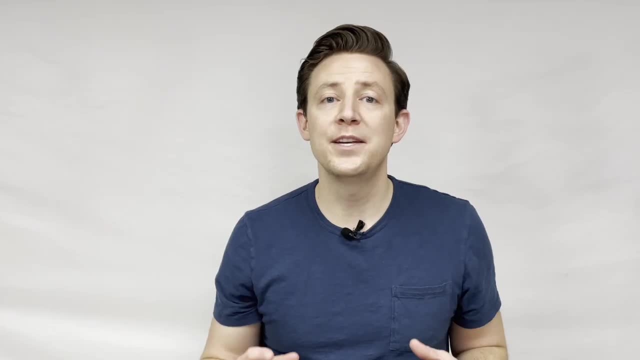 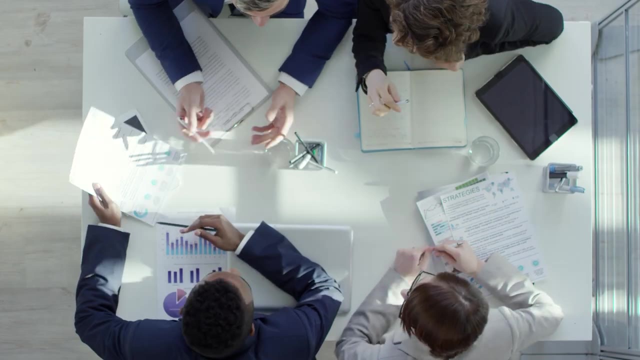 especially for lots of different roles and can be helpful across the board. But spatial SQL is really hard to learn, even in traditional settings. I had to learn this by picking up random tutorials, asking colleagues and kind of figuring it out as I go along. 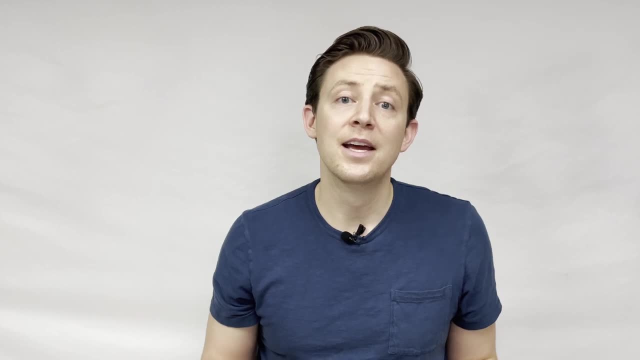 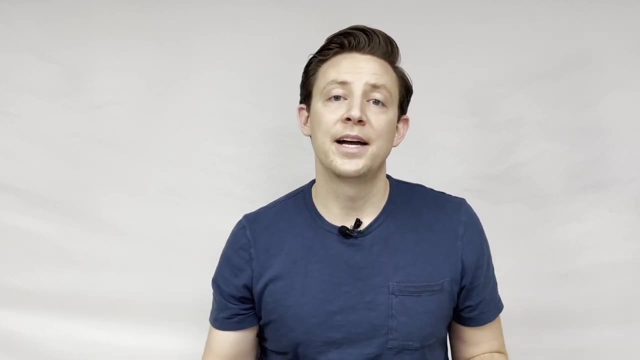 But, like I said, one of the most valuable skills that I've learned to date, And I say that for two different reasons. The first is that these functional data skills that you're going to build in SQL are highly transferable inside and outside of Geo. The second is that this really just helps. 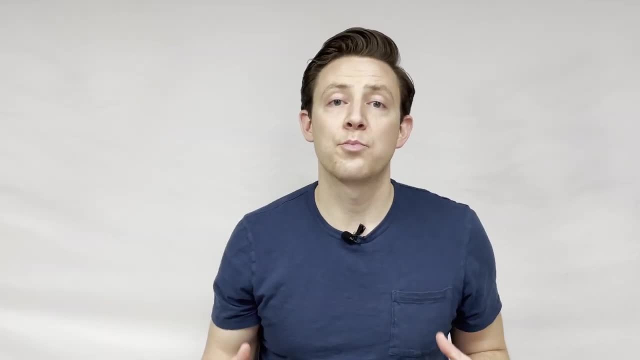 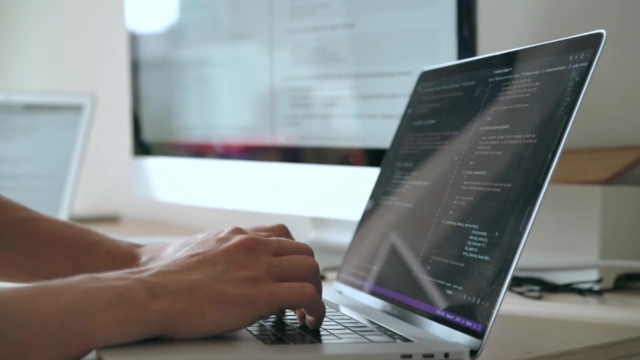 you scale up what you're already doing. This is also going to help you build really practical data skills- doing things like ETL and transforming your data- And it's also going to help you think about data in a new way programmatically. There's also a pretty low barrier to entry. 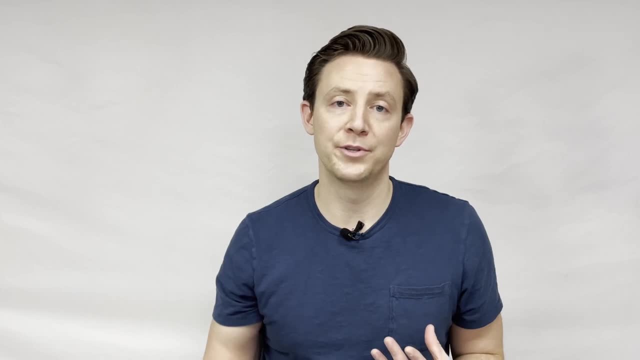 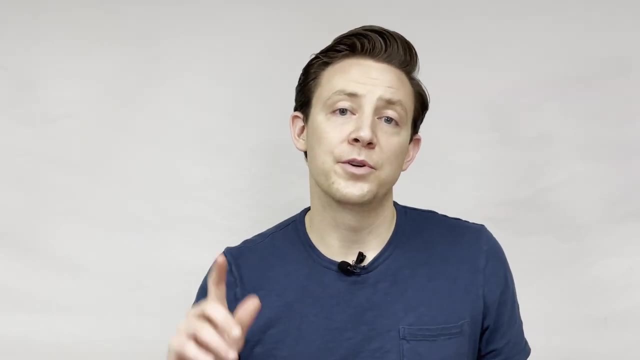 SQL is pretty easy to learn once you have a few foundational tools to do so, And you can use it as a stepping stone to different data types and other languages. I've been building a series all about spatial SQL. You can check that out in this playlist here. 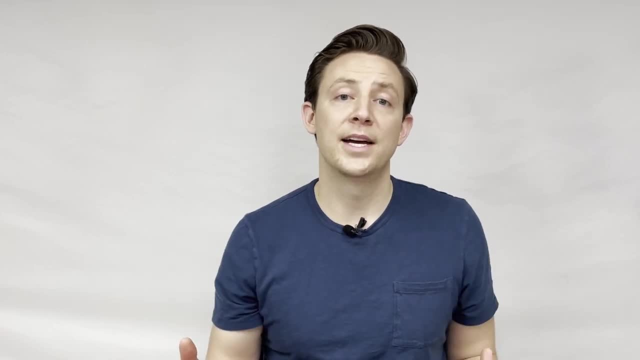 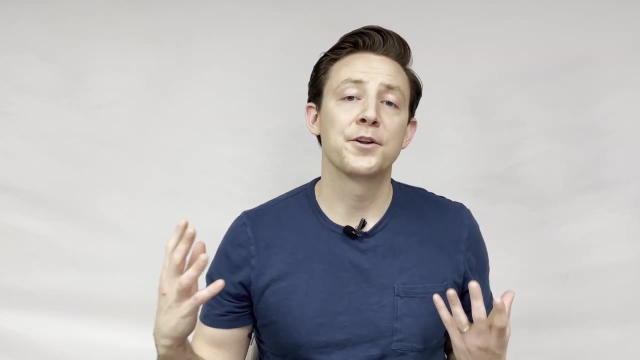 The best part is you can get started at no cost. You can download PostGIS, connect it to QGIS and you're up and running in a few minutes. Now, of course, you can analyze data to the blue in the face. Ultimately, you're going to have to create a map and visualize your data. 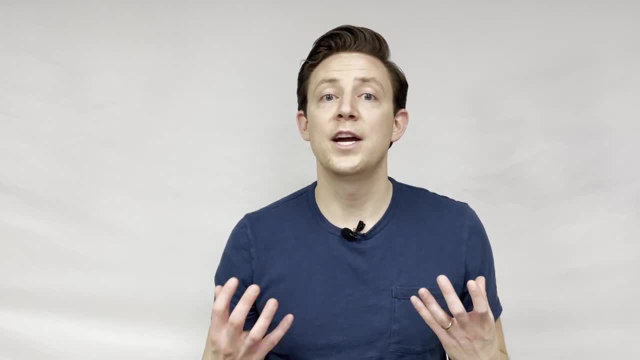 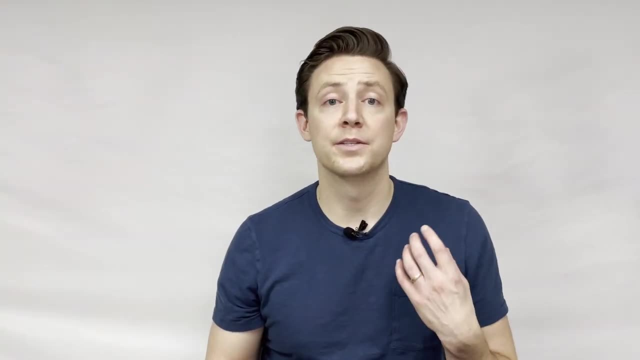 So what should your visualization toolkit look like? So there's no right answer here and there's no clear consensus on what tools you should use to visualize your data. A lot of times job postings, people asking for skills in Tableau or Power BI, But business intelligence tools just. 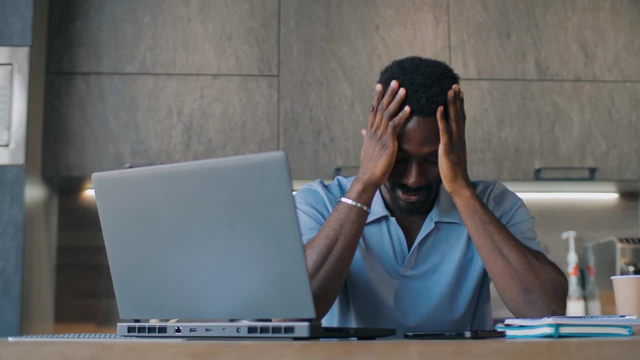 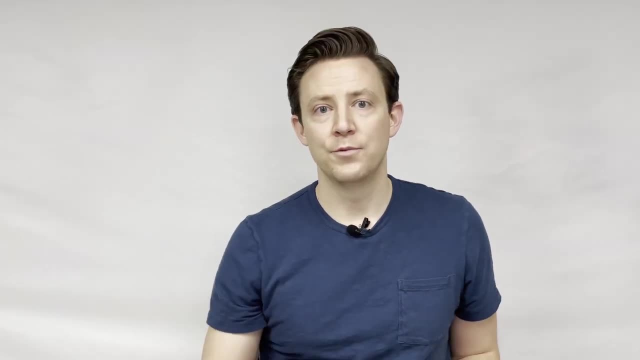 aren't suited for geospatial data. They can't handle the volume of data And once you get above a certain number of features, they're going to crash. So what are the tools that you should learn if you're focusing specifically on geospatial data? Well, the first, again, is QGIS. QGIS- lets 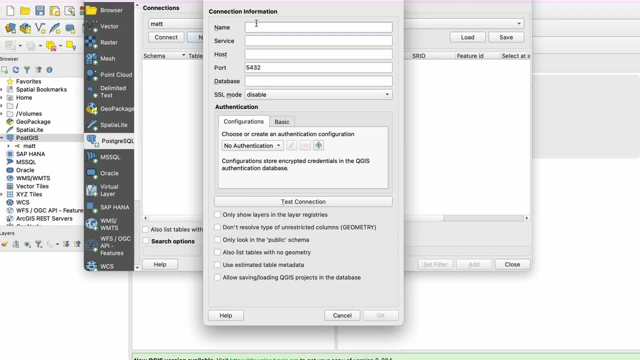 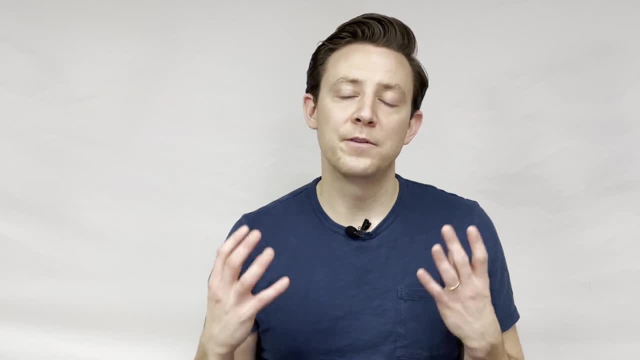 you visualize your data within the application itself. You can create map exports that are static or print versions, and you can even create some lightweight interactive maps as well. It's completely free and open source. If you're a QGIS team, this is going to be a really great way to get started, And if you're, 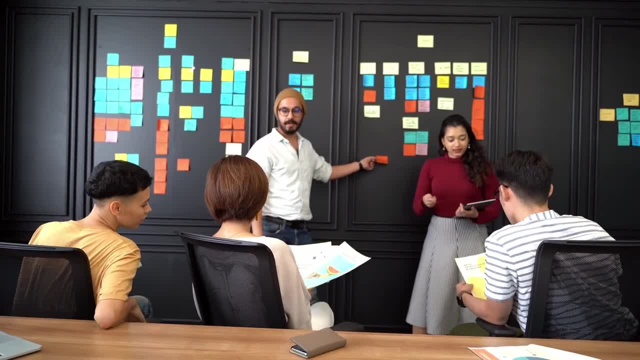 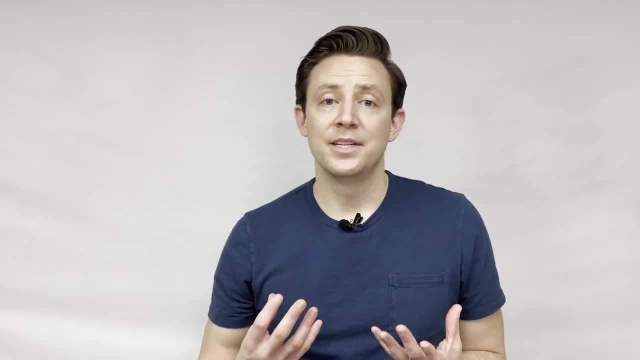 thinking about enterprise GIS. if you're all connecting to the same database, you can all share data back and forth and use that as your core data store for your team. That said, there are some limitations. It's hard to share maps and data back and forth. You have to transfer your. 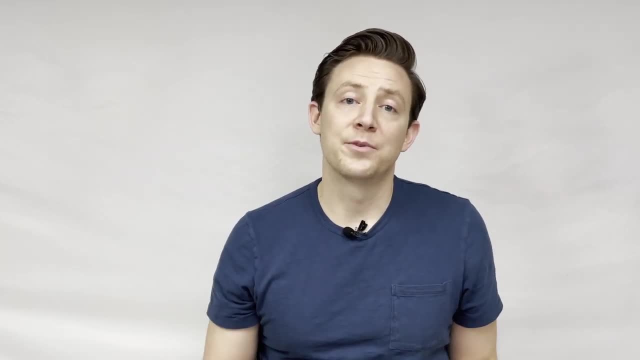 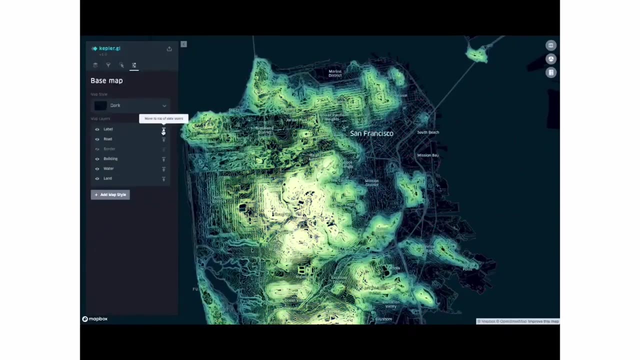 file back from one to another, So sharing becomes a little bit more tedious when you're using QGIS. The other tool I really like is called KeplerGL. This uses DECTGL as its rendering library, which is really great for the modern web. It has lots of comprehensive data visualization methods. 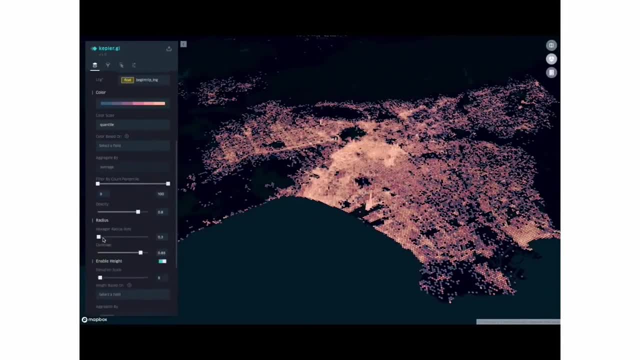 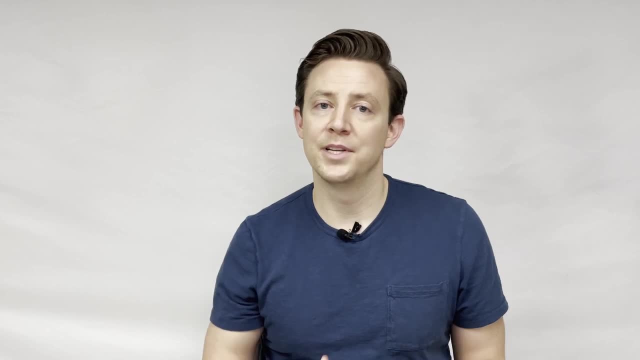 and even has some different controls to filter your data and then ultimately share and publish maps. All that said, you do have to self-publish your own maps and you also can't connect a data source like a database or something like that, So you're going to have to take your data out. 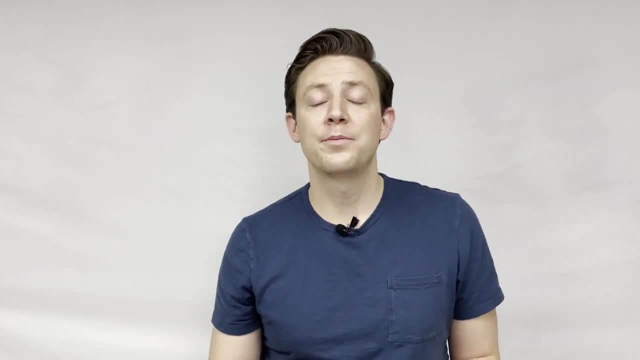 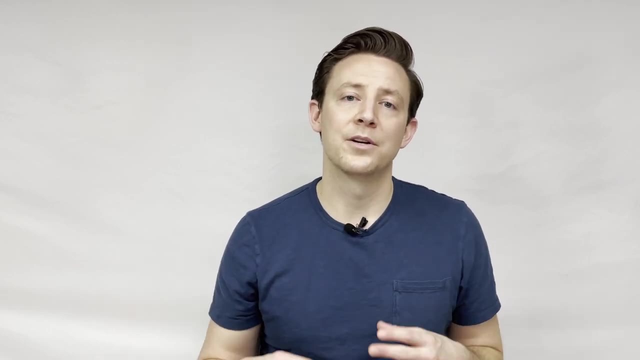 and put it back into Kepler. So those are the core limitations there. The other option is using Carto. Now, spoiler alert: I do work for Carto, so I am a little bit biased here, but I do feel like it offers some great options compared to. 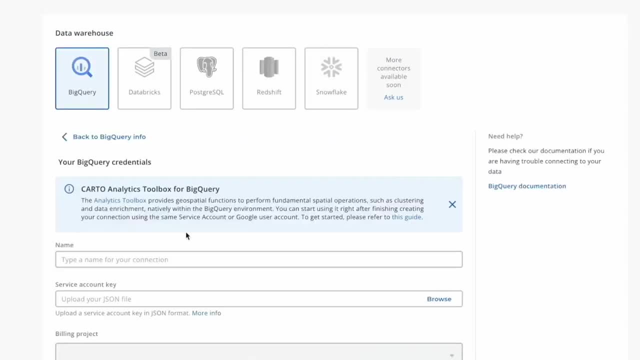 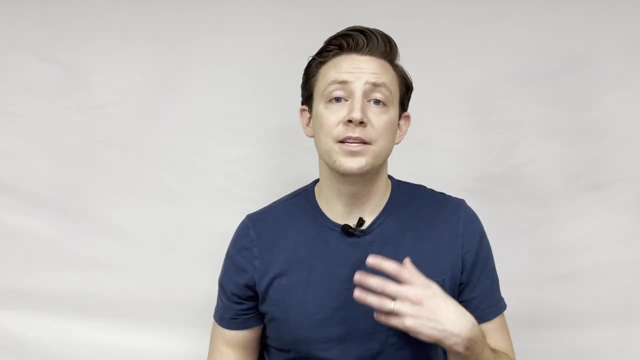 QGIS and Kepler Carto lets you connect any data source, whether that be a database or data warehouse, and you can use that to build maps, visualize them and share them. It also adds some different tools into the database or data warehouse in its analytics toolbox to make things like spatial. 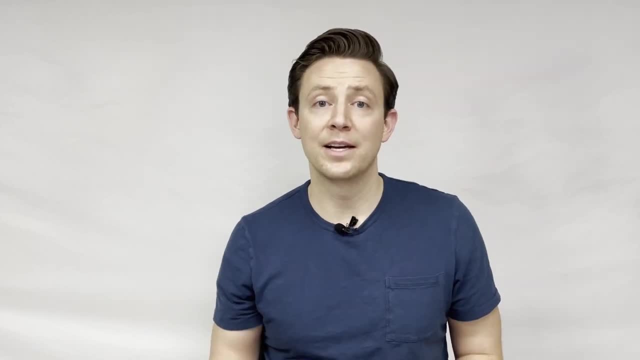 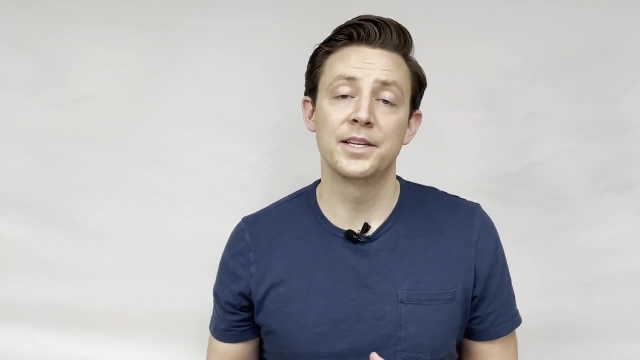 statistics, routing, geocoding and creating map tiles even easier. You can create really complex dashboards with writing, SQL or without. There are some limitations. Carto is completely cloud-based and does have a cost associated with it. If you do want to get started, you can get. 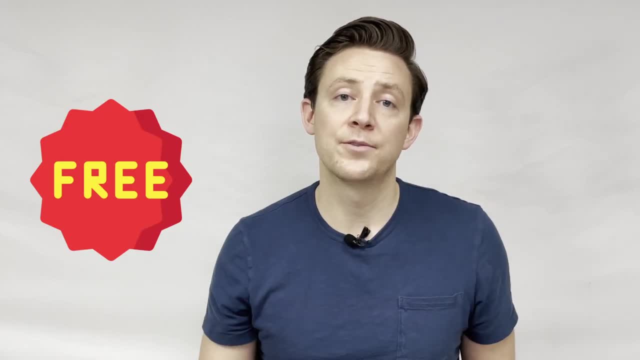 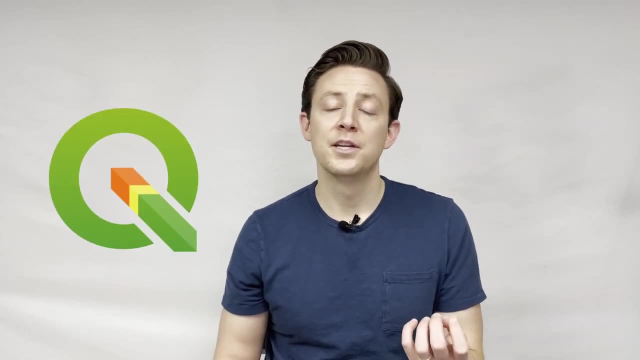 started for free with a trial, or, if you're a student, you get free access to the GitHub Student Developer Pack. There's no right answer here, but in terms of how you might start with these tools, I recommend starting with QGIS to do your base visualization and analytics And then, when you need to create an interactive map. 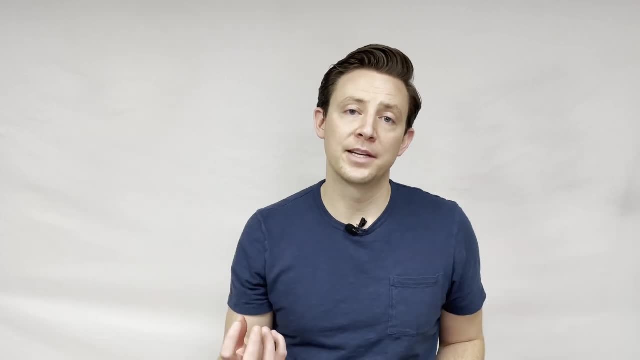 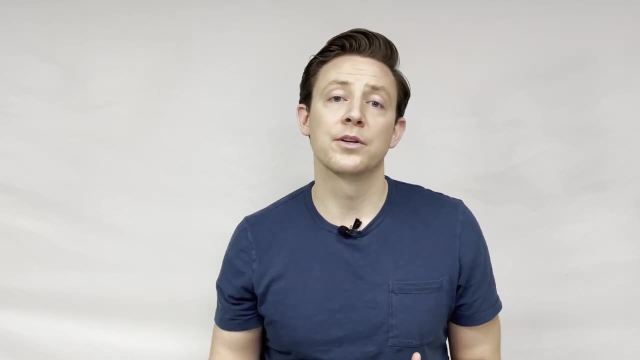 moving that into Kepler and taking your data out of QGIS and putting it into Kepler. Once you get more proficient in SQL and you're ready to do some more complex visualizations or scale up with larger data, I would take a look at Carto because that becomes a logical time. 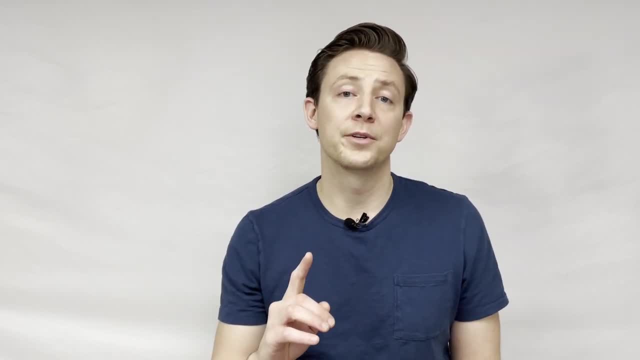 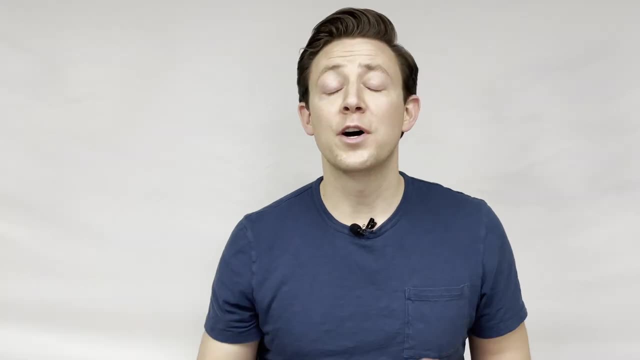 to use a more scalable tool. So we have to add one more tool to our toolkit- and you might know what I'm going to say, But it's Python. When you want to get into more advanced analytics, you really need to add another programming language to do this, And Python is the best. 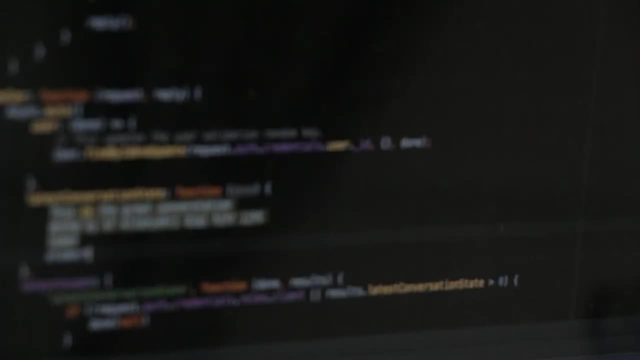 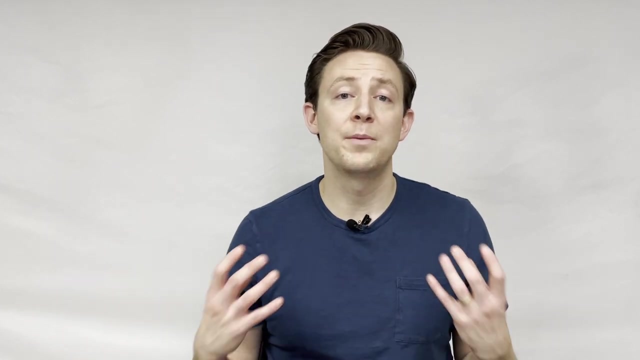 choice to do so. My first programming language was actually JavaScript, And while this taught me a lot- and I had to struggle to learn it- I wouldn't recommend that as your analytical programming language. Python is going to give you a great base to work off of and scale your skills. 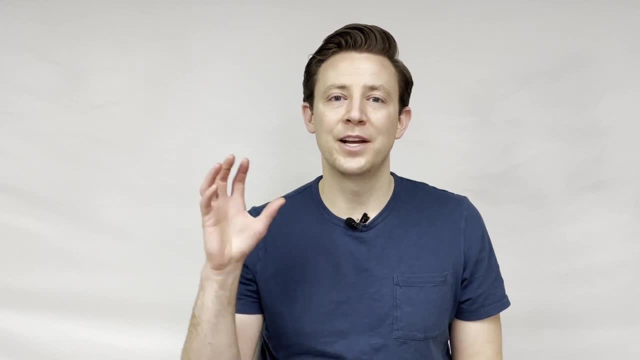 well beyond this language itself. I also get this question all the time: Should I learn R or should I learn Python? Ultimately, I would recommend Python. R is really used in academic circles And it's a really good way to learn Python, And it's a really good way to learn Python And it's. 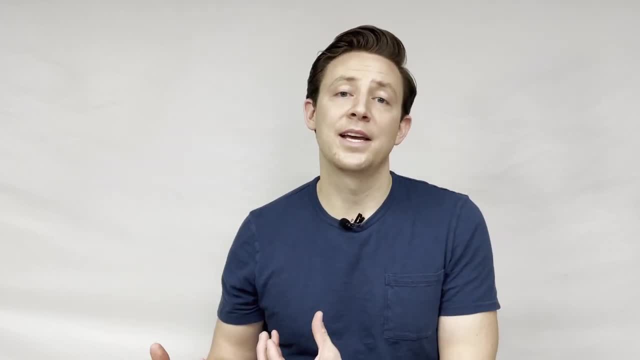 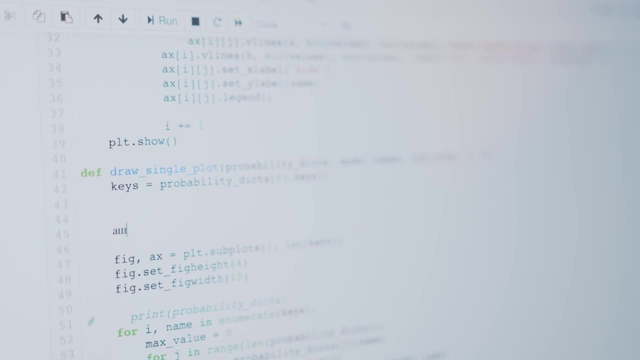 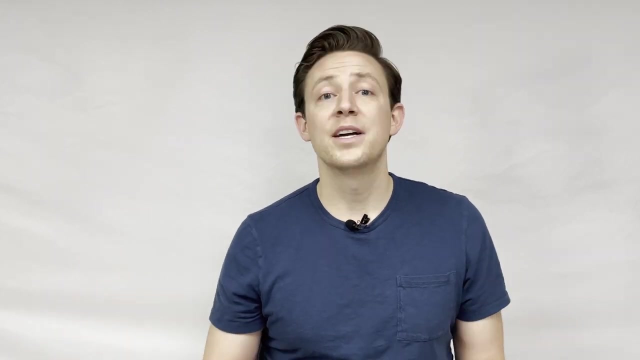 run data science notebooks, create machine learning models, even build backend APIs. It's extremely versatile, So once you learn it, you can apply it to much more things beyond just spatial analytics. Python is super easy to get started. There's a lot of courses to learn. 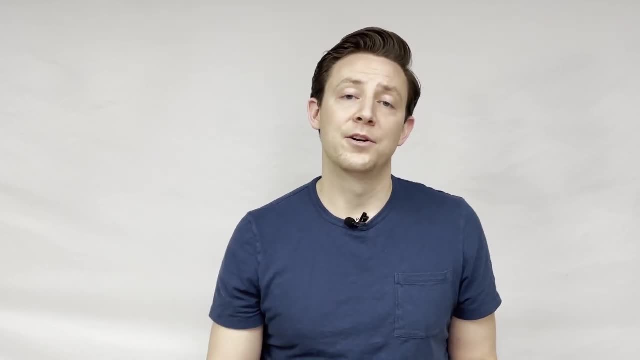 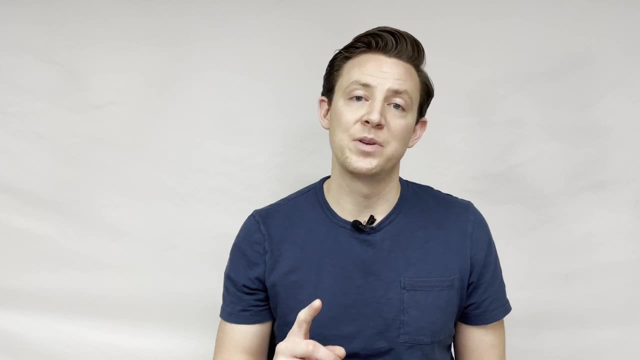 but you can take a look at this video, which has my recommendations on how to get started and learn geospatial Python. So, now that we know what to learn, we have to figure out how to learn it, And this is the first mistake that I see a lot of people make. People try. 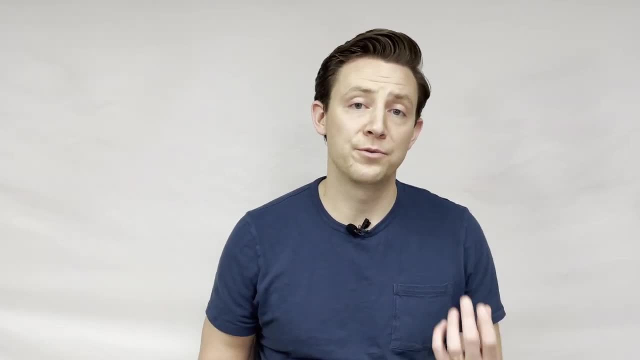 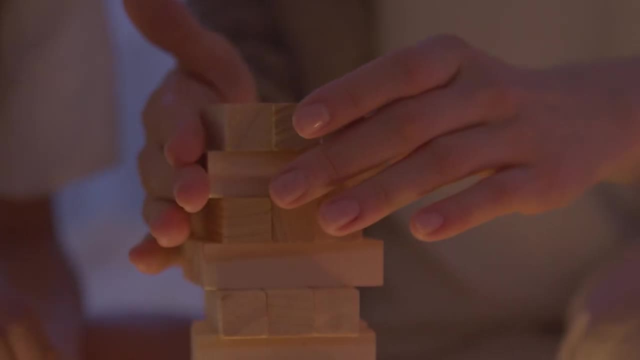 to learn everything that they can possibly learn with all these different languages and tools, And this isn't the approach I would recommend. You want to become just dangerous enough to use these different skills in practical ways And then, over time, as you pick your. 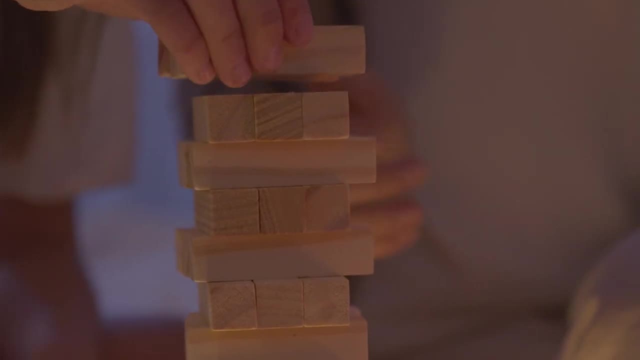 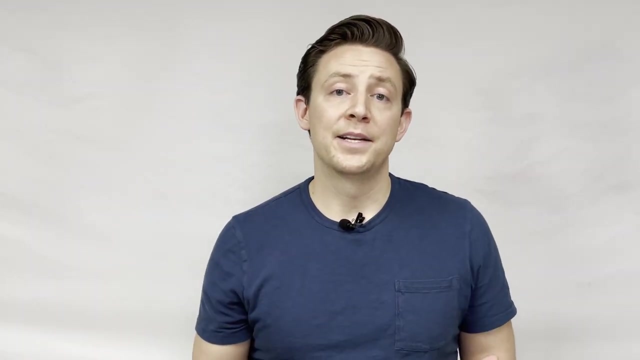 focus areas you can really start to go deep. If that's in spatial data science with Python or in data engineering with SQL, you can really figure out where your interests lie. The other problem with this is that people spend a lot of time watching tutorials, and I mean really. 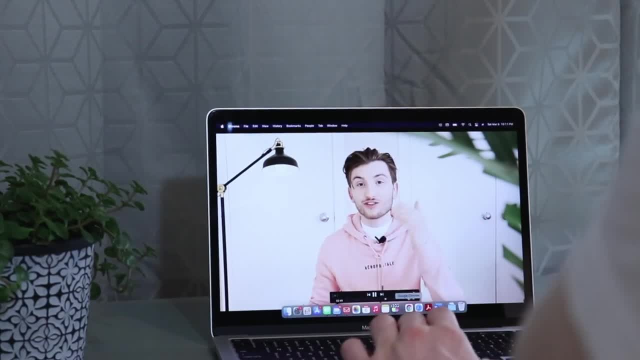 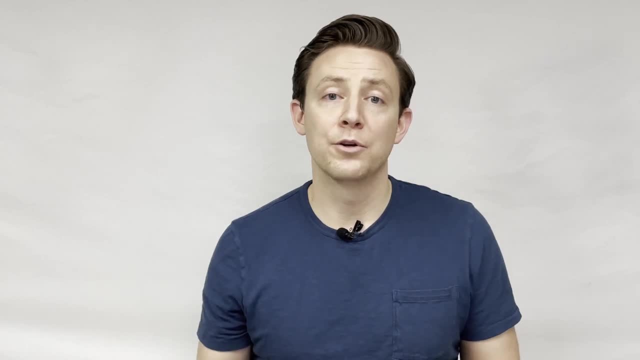 watching them. The number one thing that I find really interesting about this is that it's really easy to get started. The first thing that you can do is actually practice writing code, even if this is a simple hello world statement or building your skills over time. If you're practicing writing code, 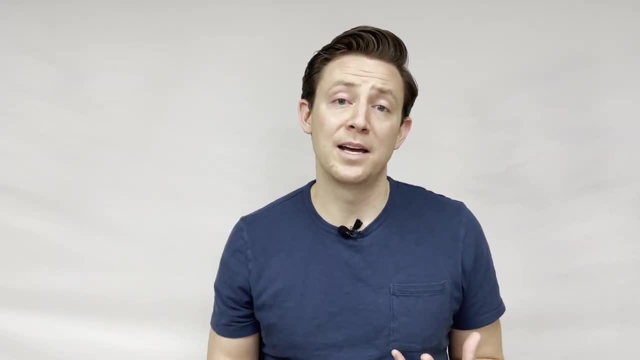 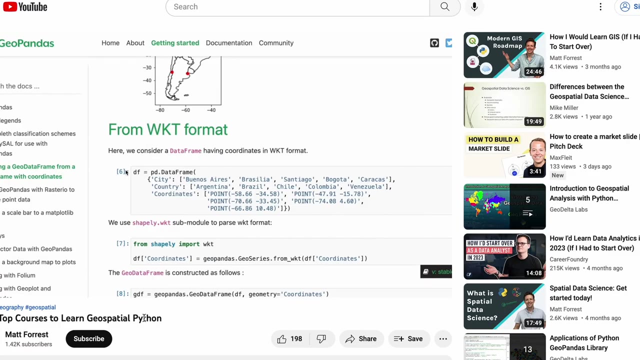 you're building your skills. Courses are really great and I've learned a lot from them over time, but there's a lot of great free tools out there that help you get started and actually have practical exercises to do this. I shared this earlier in my videos for geospatial Python. 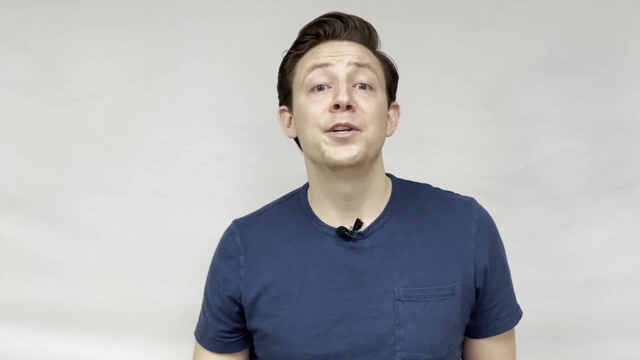 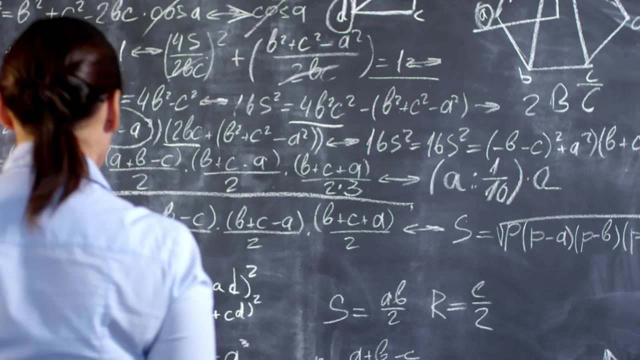 and the first video on my spatial SQL course as well. The other thing you need to know is analyzing geospatial data in practice is way different than watching it. So getting your hands dirty, Hitting some walls and trying to figure out problems is the best way to go, Knowing how. 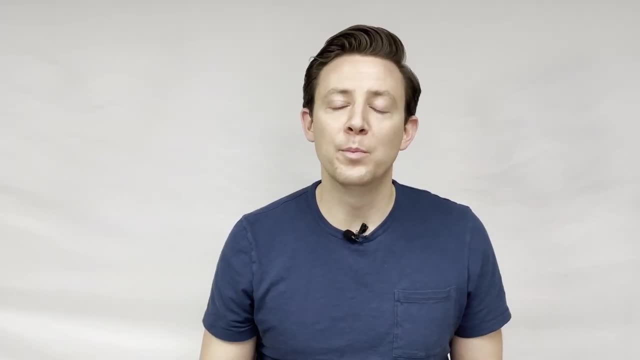 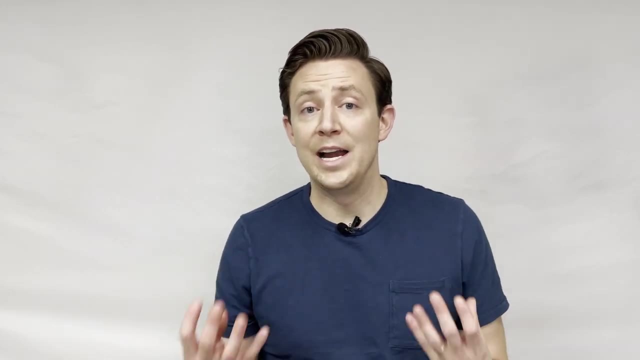 and what a spatial join is is way different when you have to join a couple million points to a couple hundred thousand polygons. What's the best way to practice? There's a few things that I can recommend. The first is to design your own challenges You can actually think of. here's a problem I want. 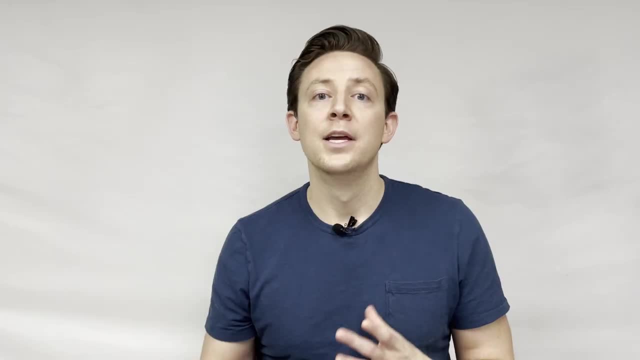 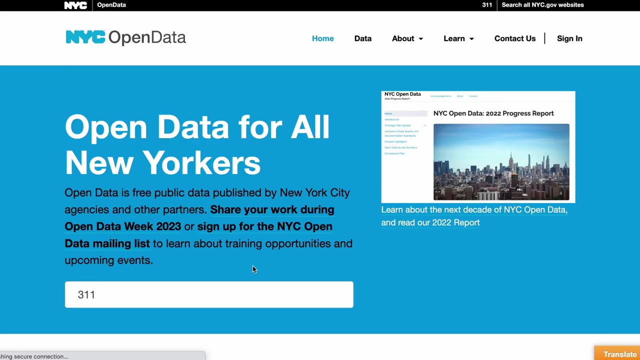 to solve, and how would I solve that? with Python or SQL and decide how you want to go from there. There's so many great open data sets to test this out. Basically every city or country in the world has an open data portal, so you can go and grab some data and start. 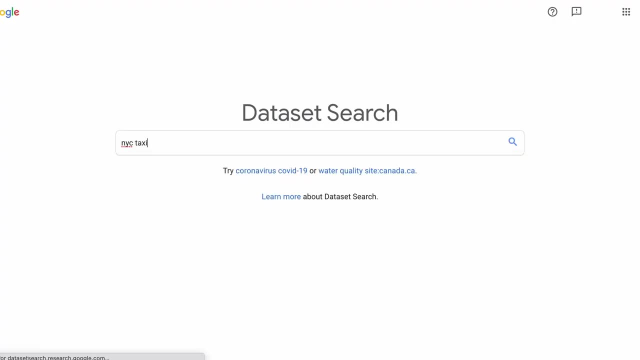 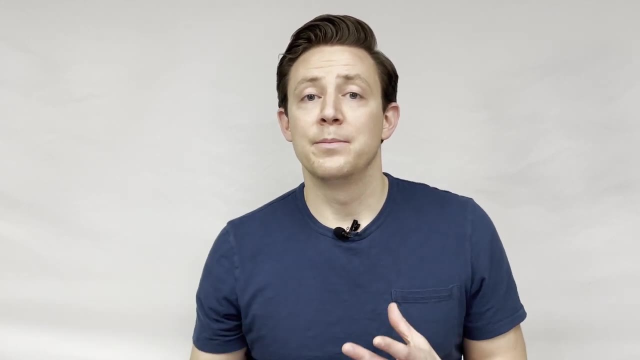 solving different problems. that way, You can also look at different data sources like Google open data as well, as there's lots of geospatial data sets on things like Kaggle and other places too. Another great way I recommend is looking on medium and trying. 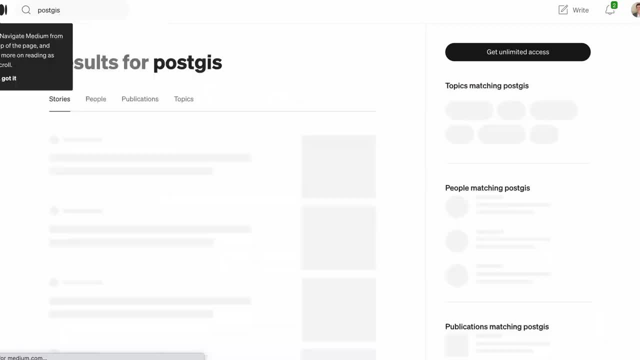 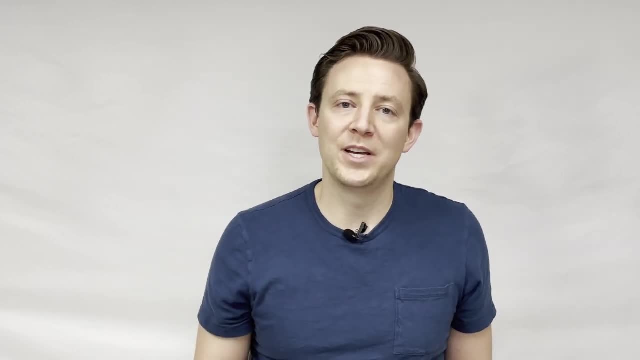 to find projects that you like and find interesting and replicate them or add a different spatial angle to them. Find three, maybe four projects that you really find interesting and take your own spin at them from a geospatial perspective. I'd also recommend investing, maybe in a few. 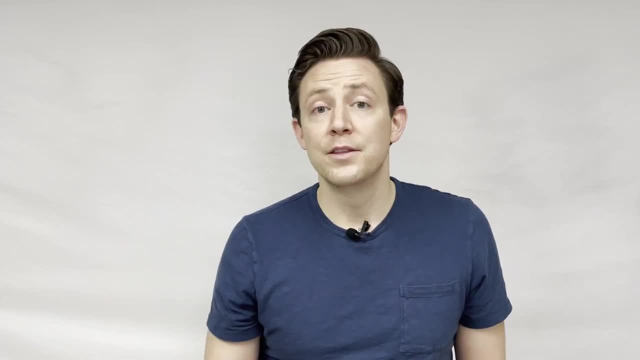 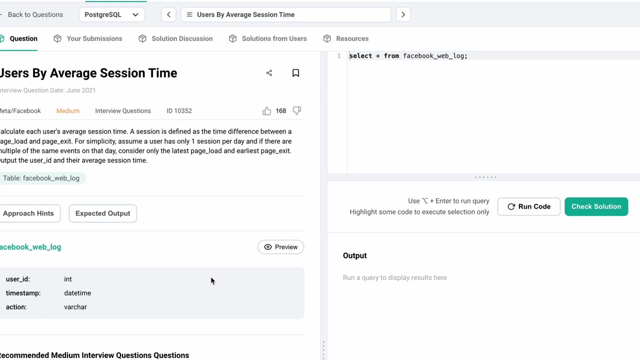 different training tools that are specifically focused on helping you practice. There's a few that I really like: Stratoscratch: It's built by data scientists and actually puts you into programming challenges for SQL as well as Python If you're focusing purely on SQL. LearnSQLcom is another awesome resource. 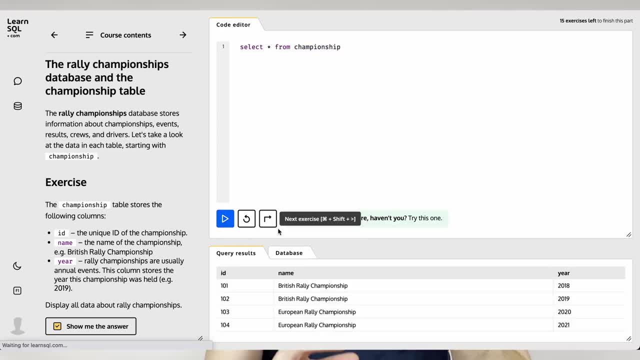 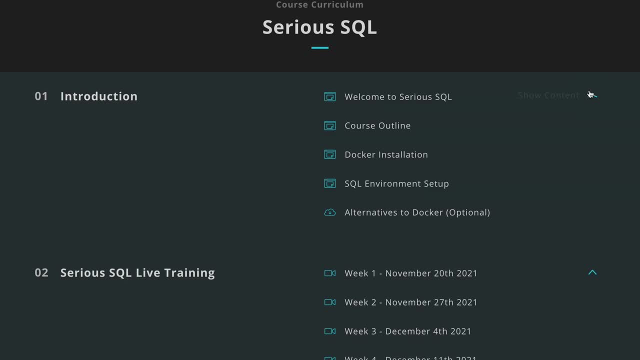 that I really like. There's lots of tutorials. You can take everything or just the bits that you want to focus on. The last one is Data by Danny. If you're going deep, deep, deep into SQL, this is the best route to go. There's an eight week SQL challenge that he has as 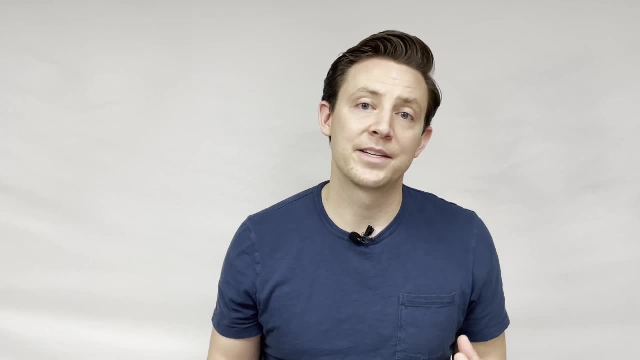 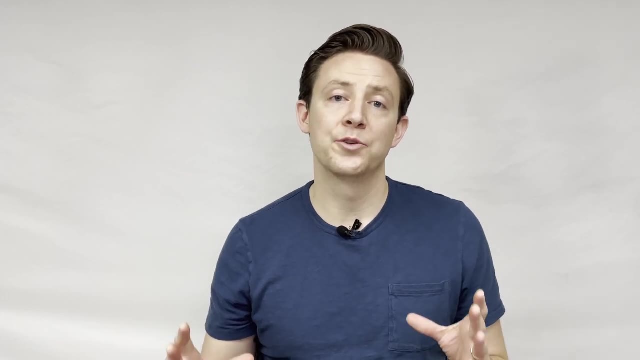 a complete course that really focuses on deep and intense topics. You can do all of this totally for free, with no cost, but if you're going to invest in a tool, I would definitely recommend it. I would definitely invest in one that gives you actual problems to work on and train. 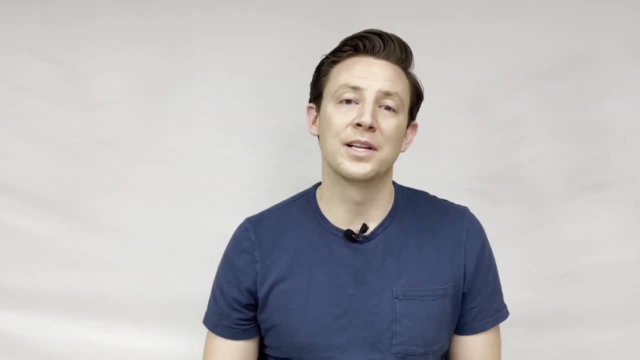 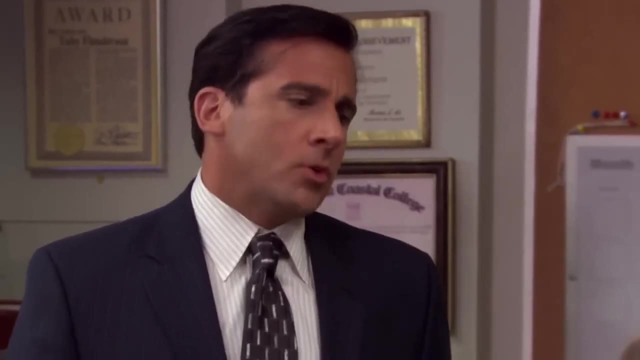 The second biggest problem I see people make is feeling like they have to figure it all out by themselves. Guess what You don't? In analytics or geospatial analytics, something is inevitably going to go wrong. No, God, please, no, No, No. 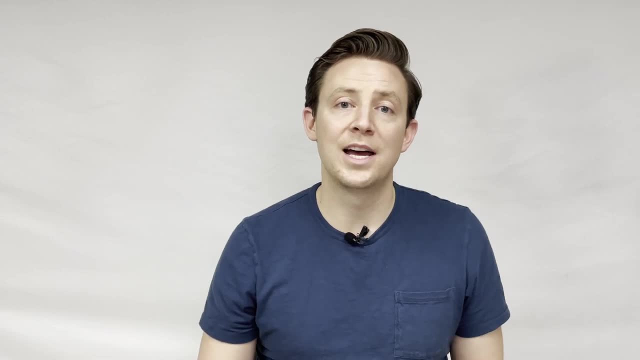 And you're going to have to figure out how to fix it. This is where you're going to spend a ton of your time working in technology. no matter where you are, You're inevitably going to end up on Stack Overflow at some point trying to figure out how to do something. 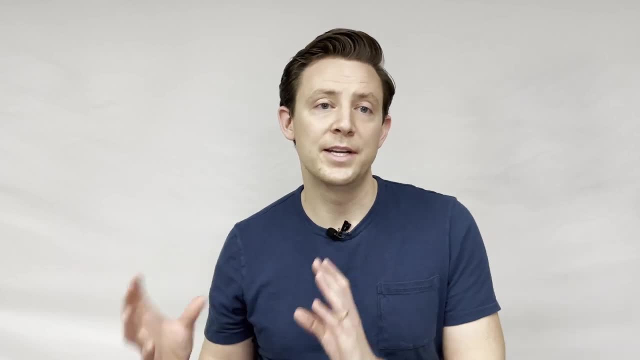 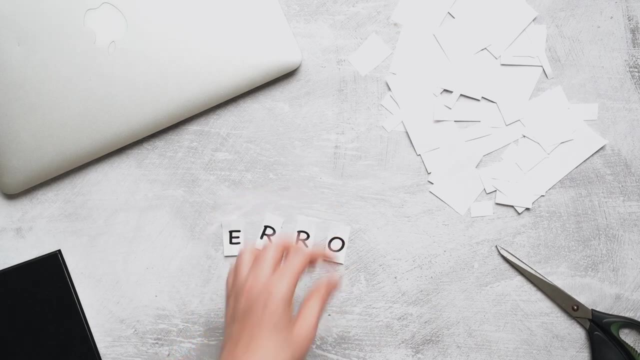 My other advice is to learn how to read error codes. Error codes can be super annoying, but a lot of the times, if you can read them and understand what the problem is, that might give you a clue as to where the problem might be. 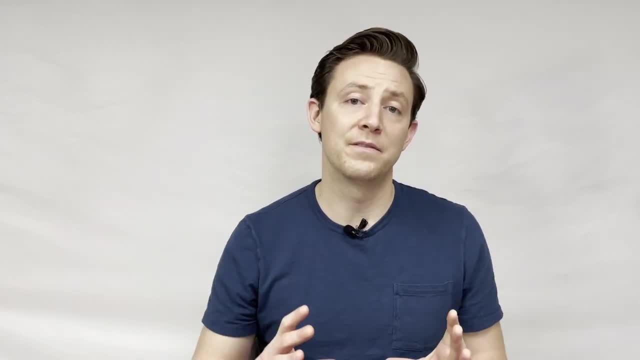 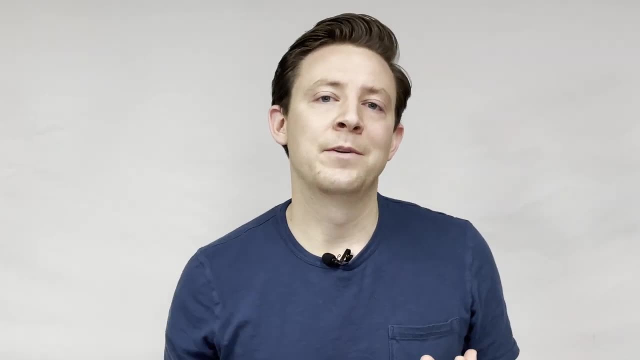 And also reading documentation to see what needs to go into a function and what comes out of it, is going to be a valuable skill as you start to get deeper and deeper into these tools. So now we've picked our tools, we've learned them, and now it's time to find a job. 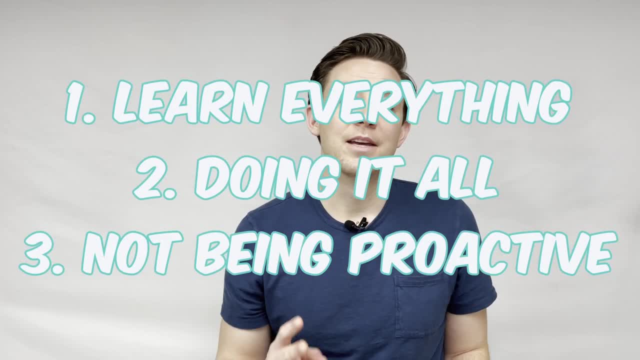 And this is actually where I see people make the third most common mistake, and that's not being proactive. What do I mean by being proactive? It's actually three things: First, building your portfolio. Second, building your business. Third, building your business. Third, building your business. 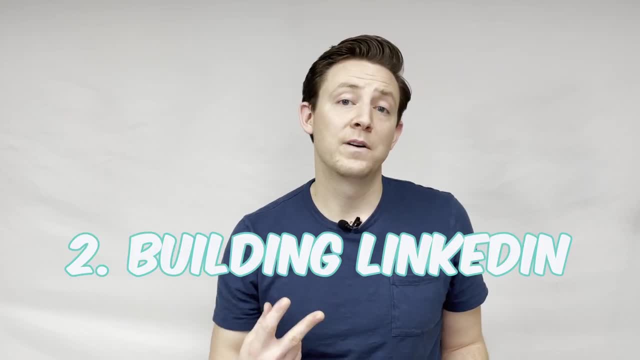 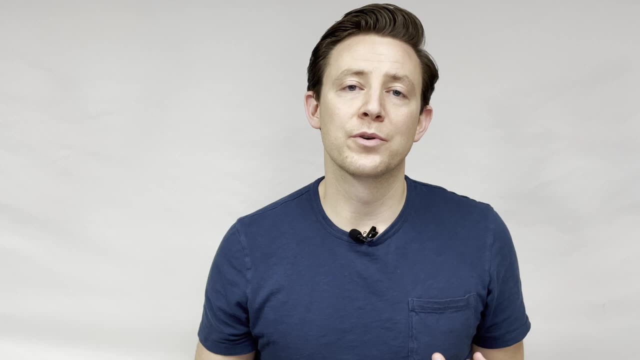 Second, creating and building out your LinkedIn profile. And third, reaching out to people that you might want to work with. So the first step is building out a portfolio. Why is this so important? Building a portfolio shows that you, first of all, know how to do the work, but also 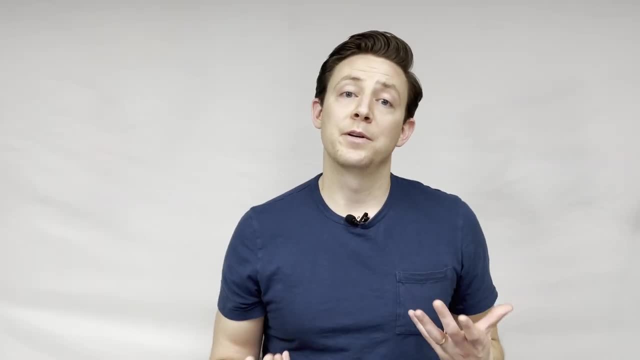 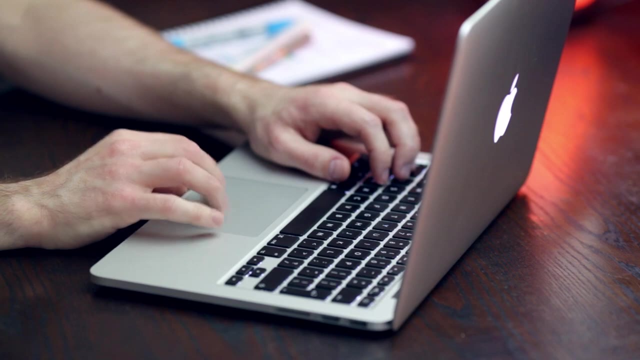 that you've actually had some practical implications for this. So how do you start building portfolio projects? If you can actually do this in your current job? great, That's a great place to start and actually apply your skills and build some different projects. If not, try to find some. 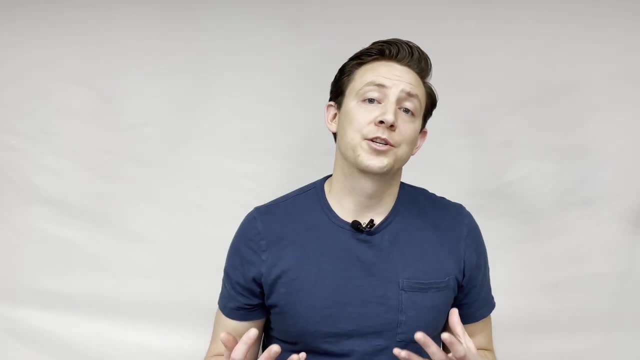 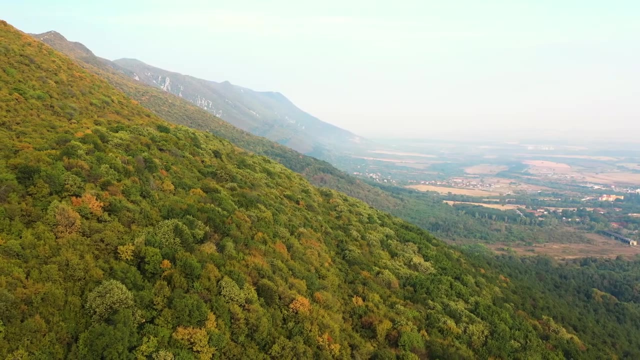 projects or some passion projects. No matter what the project you do, make sure it's unique to you and you're passionate about it. That's going to shine through, no matter what that is. If you're really passionate about the outdoors, do something with national parks data and try to figure out which parks 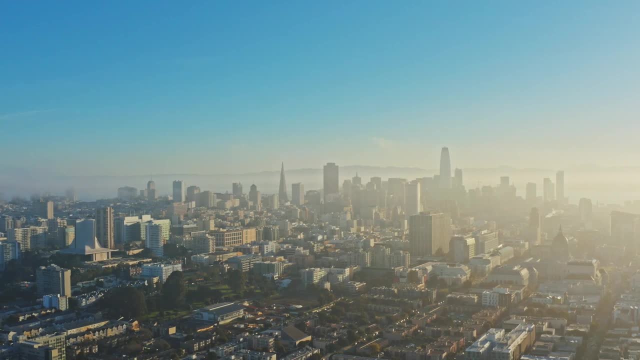 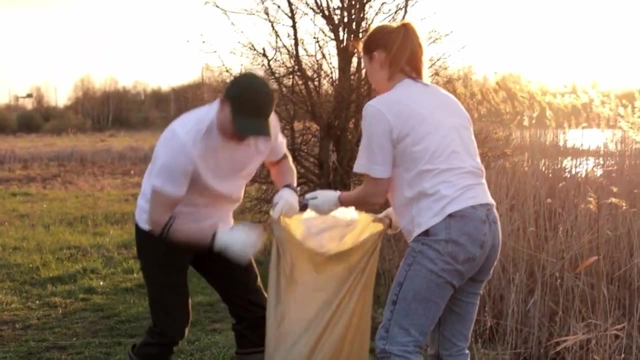 have the most visitors. Are you passionate about cities? Great, Go, find some open data and build a project there. Another tip is you can even reach out to nonprofits or businesses. figure out if they have a geospatial problem and actually help solve it for them. You can start this for free or turn into a 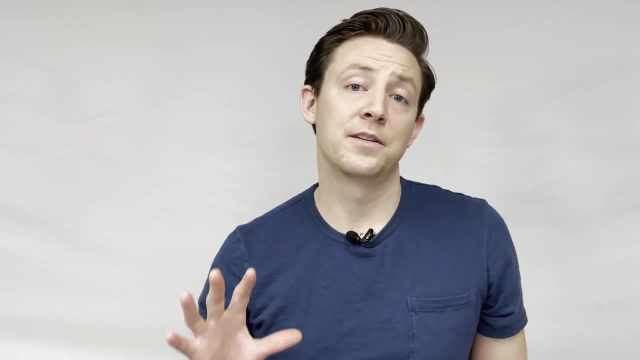 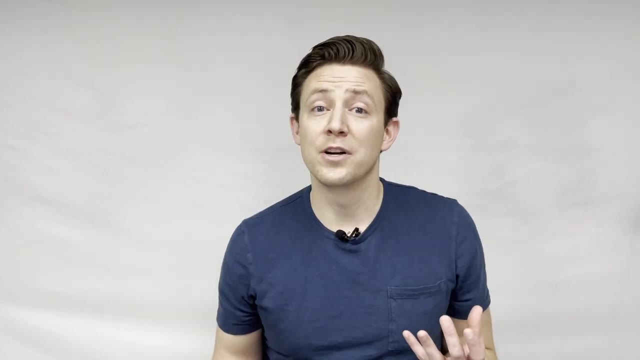 freelancing side hustle as well. I'll go into portfolio projects in a future video in far more detail, but just getting started is the most important piece Now. where should you put your portfolio, Frankly, anywhere? Building a simple website on WordPress. 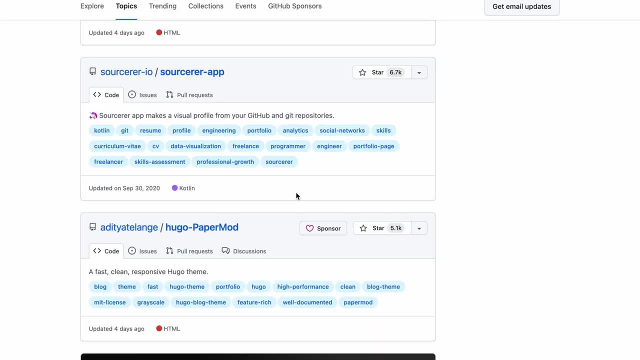 or even a simple HTML page is one way to start. Make sure you get your work on GitHub. If you're hosting code, this is a great place to go, And also check out Spatialnode, which is a portfolio tool just for the geospatial community. 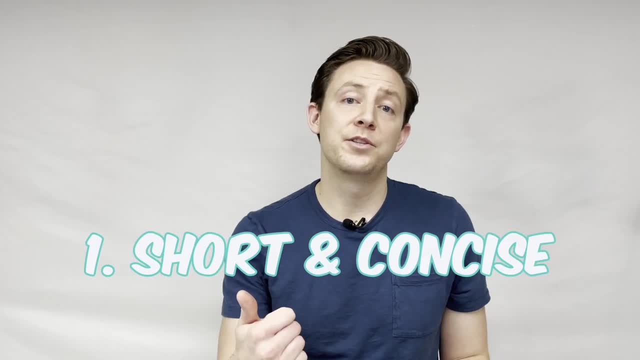 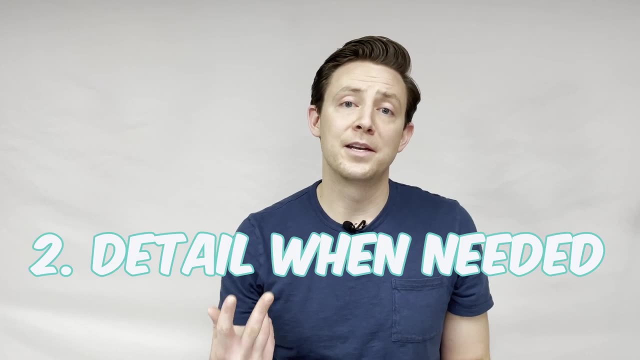 When you present your portfolio projects, they should have three things. They should be short and to the point. They don't need to go into pages and you don't need to have a 50 page report about them. All that said, They should have some detail in it. Talk about what you did, how you did it and what were. 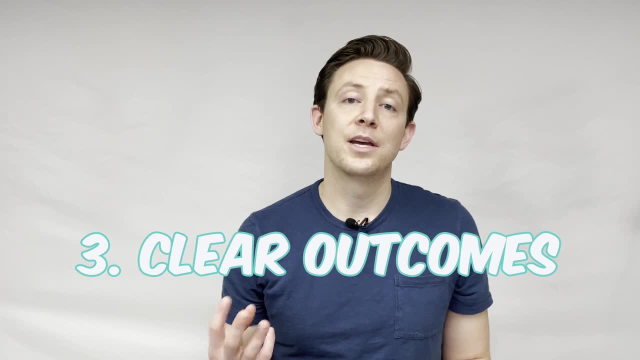 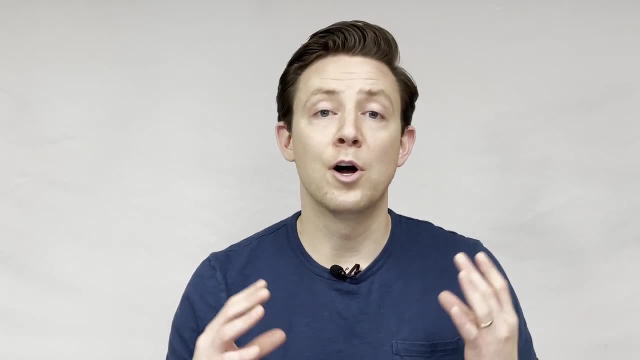 the outcomes, And that's actually the third point. What are the outcomes and what did you solve? Did you find a new trend? Did you uncover something in the data? Focus your point on that. Outcomes are the focus of all geospatial analytics, So make sure you put that front and center. 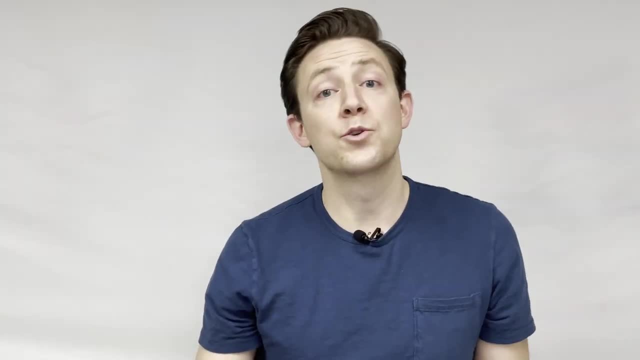 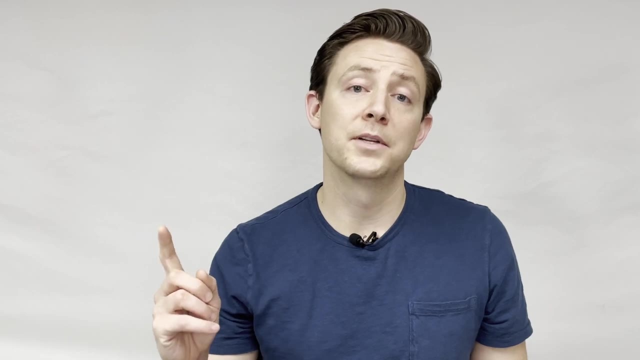 Now it's time to move in and optimize your LinkedIn. How do you do this? There's great resources on how to optimize your LinkedIn to get a job. I actually really liked this video that tells you a lot more about creating a really effective LinkedIn profile You can. 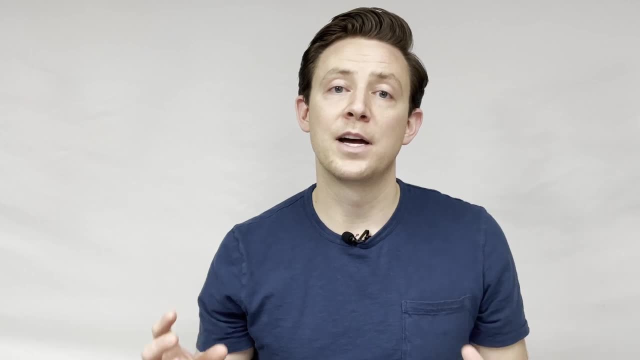 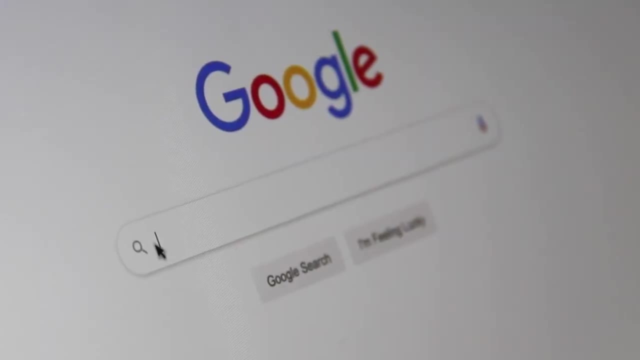 start using keywords and adjusting key components of your profile to help you find a great job that's going to be a good fit for you. In general, try to think of LinkedIn as a search engine. If you want to become a geospatial analyst, put that in your headline in different parts of your profile. 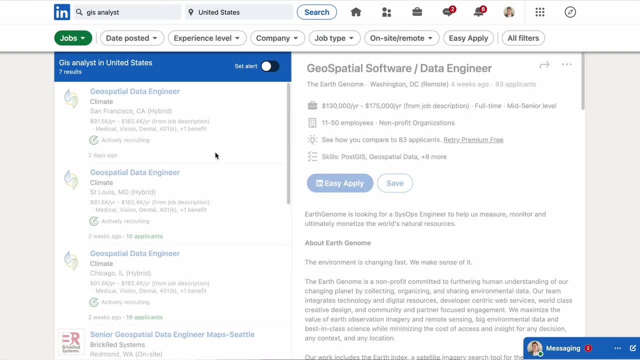 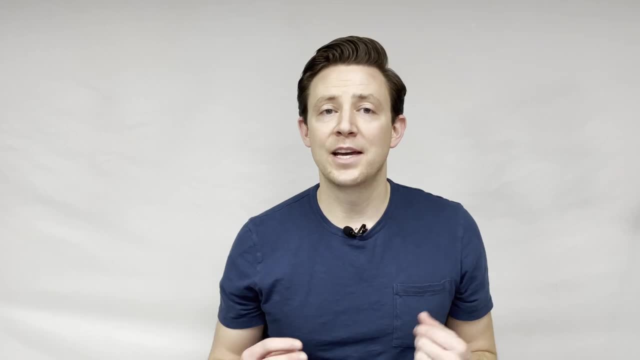 Or you want to be a geospatial data engineer. Great, Focus on that and add the relevant skills Now. in a perfect world, you build all this and recruiters start reaching out to you, But unfortunately, in geospatial, you can't always count on that. 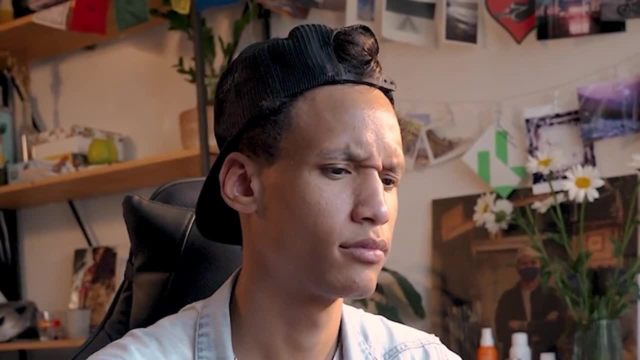 Geospatial is still a niche and lots of recruiters, unless they're working at a company that's really focused only on geospatial analytics, are not going to be able to reach out to you. Don't always know the right things to search or search for. 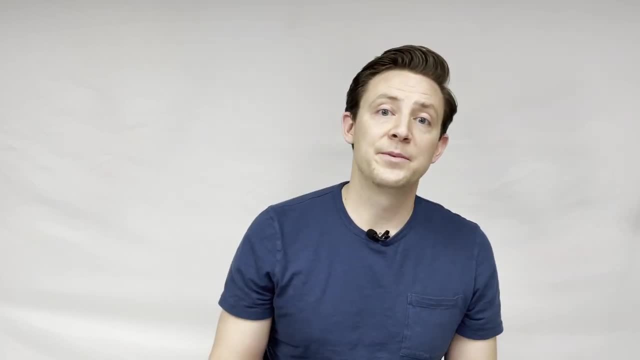 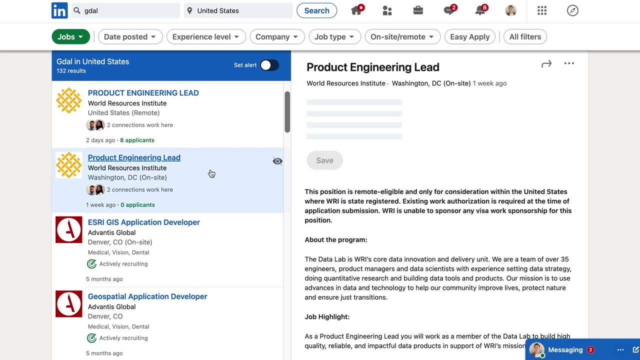 It's up to you to first of all look for roles that might be a good fit. Sometimes in a data analyst profile, you might find a listing for someone who wants to build maps. Are you looking at data engineering? You might actually learn that they might be using GDAL. 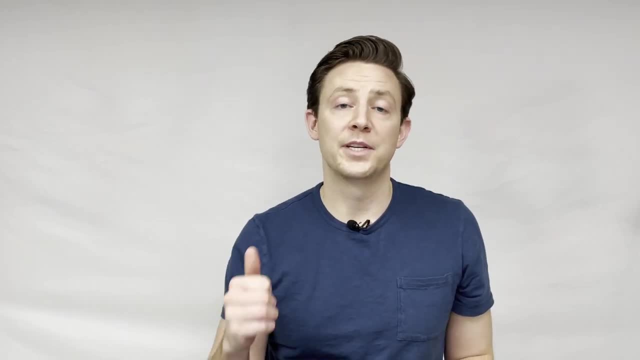 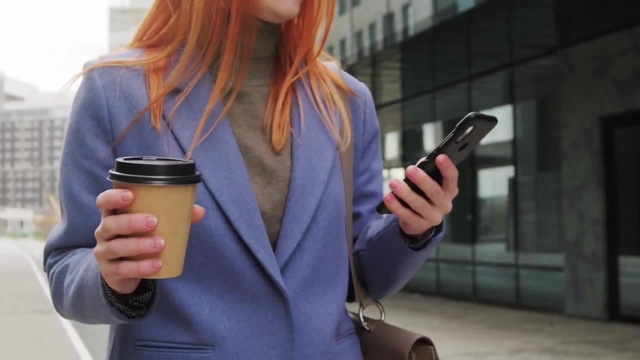 and that's a great way to search for that. Here's another post to actually search for different terms and optimize your searching when you're looking through job listings themselves. All of this is great, but the number one tip I have for LinkedIn is being proactive. That 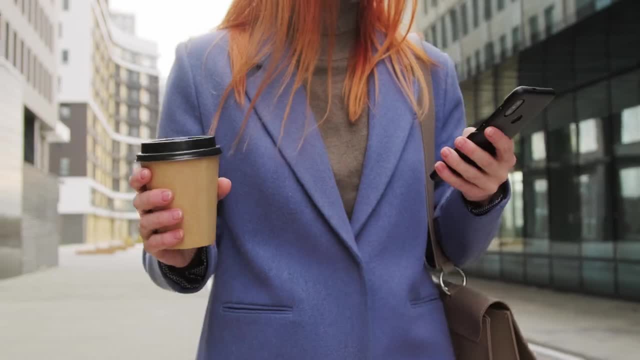 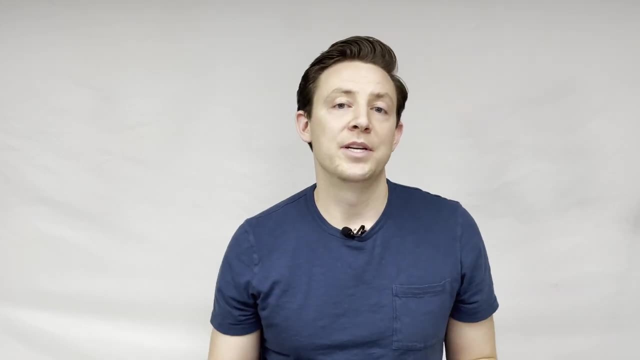 means sharing your ideas, posting about things you're learning, posting your portfolio projects and, most importantly, reaching out. Geospatial has one of the most active and engaged communities on LinkedIn and other social platforms, and people are always learning from and sharing with each other. 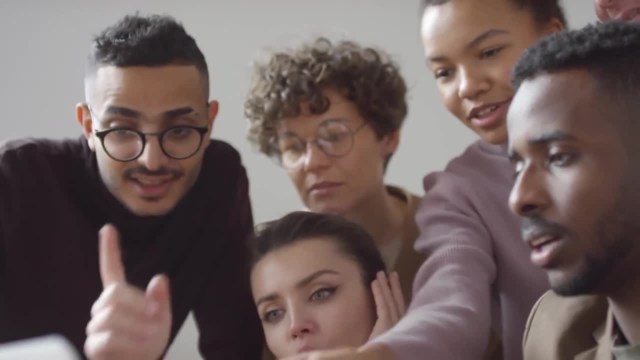 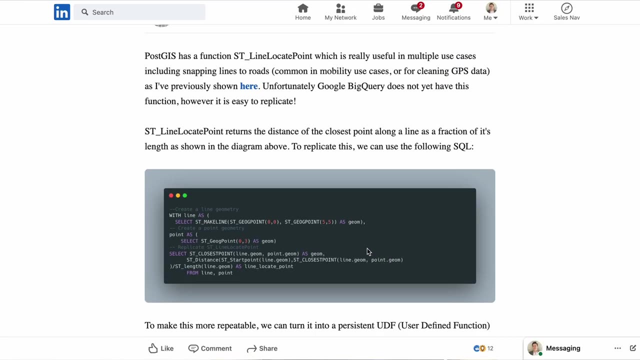 Take advantage of that, Jump into the conversation and share interesting things that you see, you're working on or you're excited about. Did you build a great new portfolio project? Great Share it. Did you find a new code snippet that was really helpful for you. 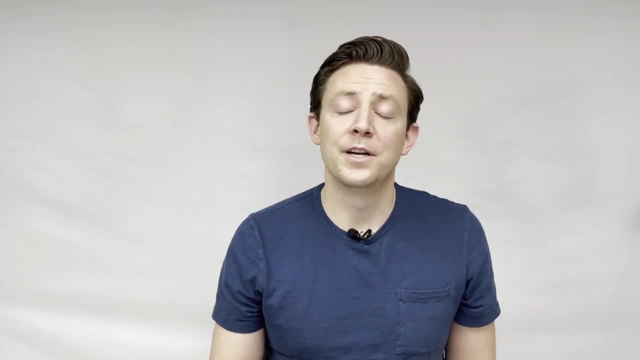 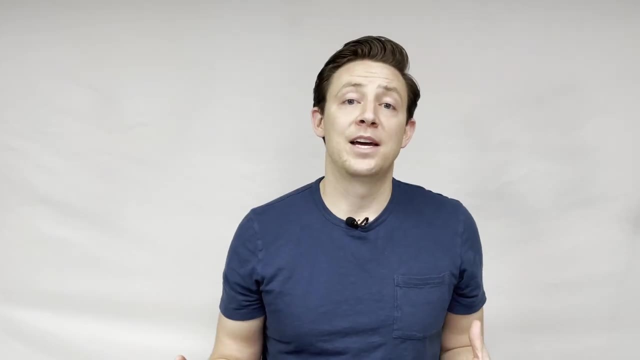 Great. Share that with everyone as well. The other thing I would say is: don't be afraid to reach out to others. If you see someone that's working in a team or a role that you're particularly interested in, reach out. It might not work out the first time. 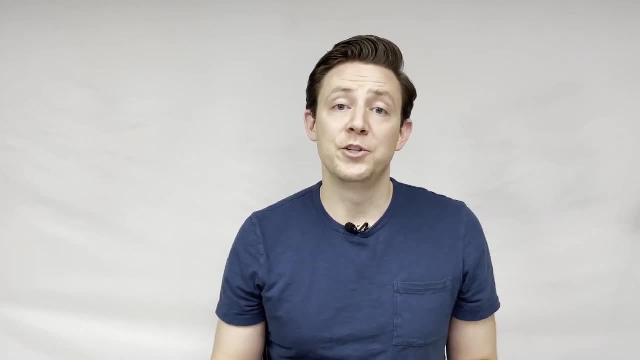 but they might have something in the future or they might know someone who is in need of a geospatial expert, like yourself. Give it time, keep up the hard work and eventually it will get there. Now, in a lot of other spaces. 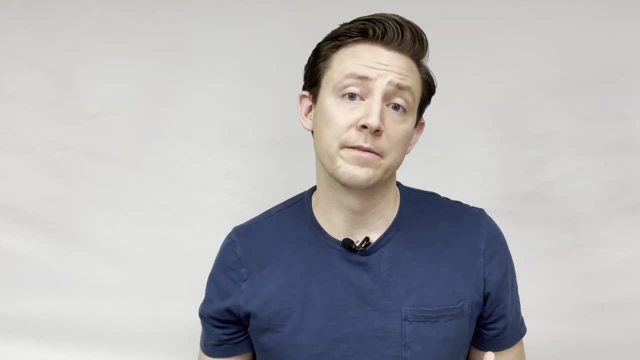 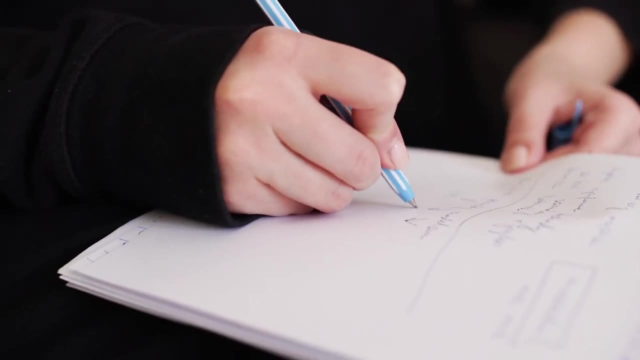 you'll see a ton of emphasis on the technical interview or programming of interviews. Geospatial interviews vary widely, so what you want to do is be able to ask questions, and any information that you can get beforehand is going to be really helpful for you when you jump. 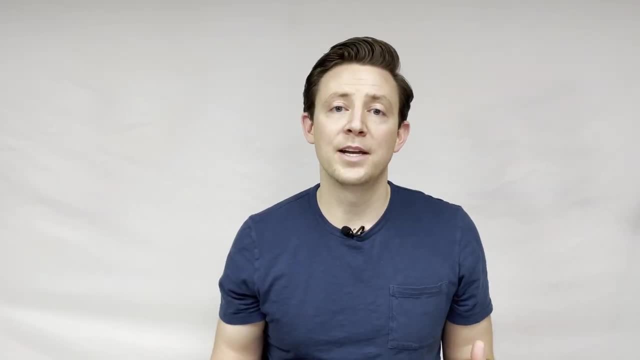 into those first interviews. If you had a tough interview or something didn't work out- great, figure out what to do next. If you have a tough interview or something didn't work out- great, figure out what that is and try to change it for next time and reimplement it. Keep practicing. 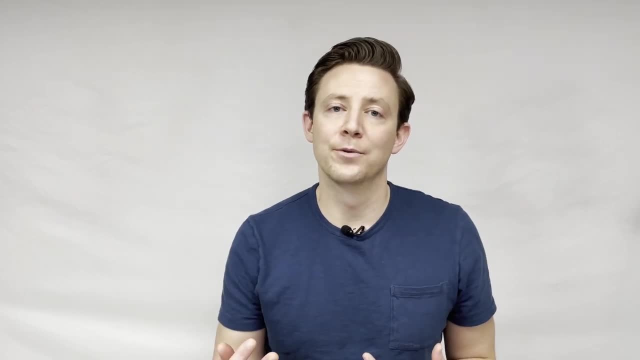 keep trying and eventually you'll translate that into success in the real world. Geospatial analytics is booming, so now is the time to jump in with two feet: start learning, growing and building your career.